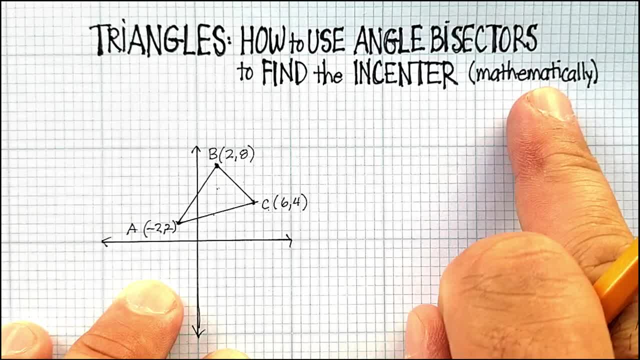 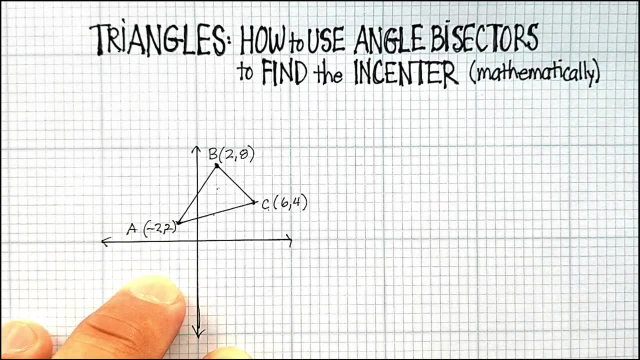 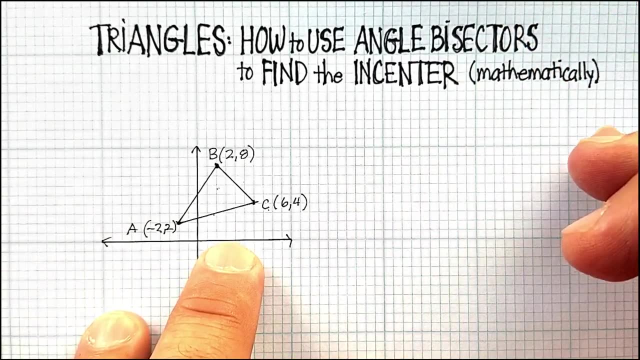 by measuring the angles and then just doing it that way, or we can do it mathematically, and that's what the purpose of this particular video is. So let's go through the steps to find the in-center of a triangle mathematically. Okay. now there is actually a formula for this. 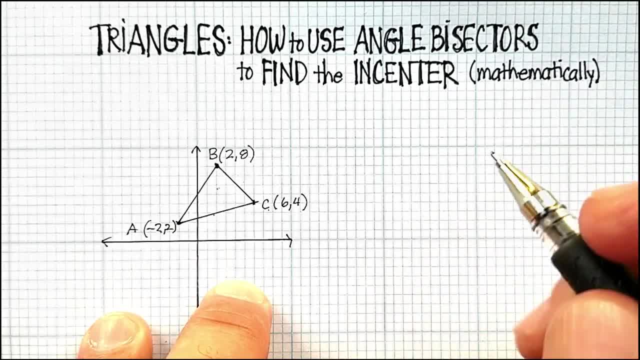 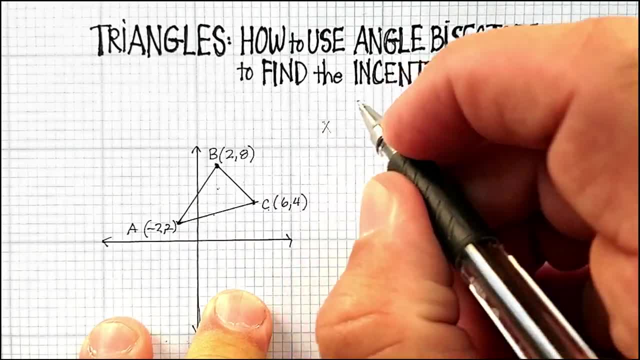 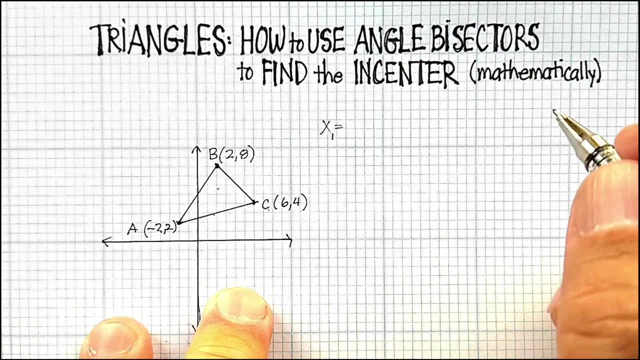 and let me just go over the formula for it. The formula is the x, let's just say it's approximately there. The x coordinate or the x point will be equal for the orthocenter or, excuse me, for the in-center. I'll just go: x sub i is equal to. 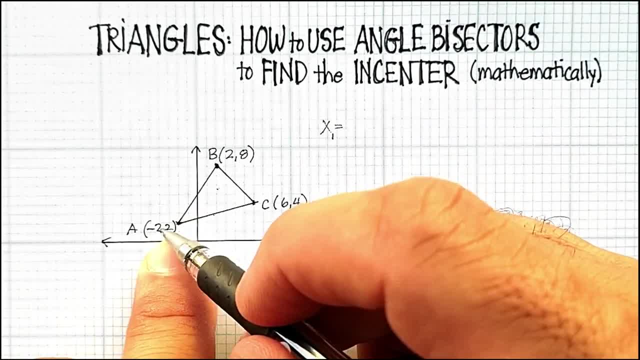 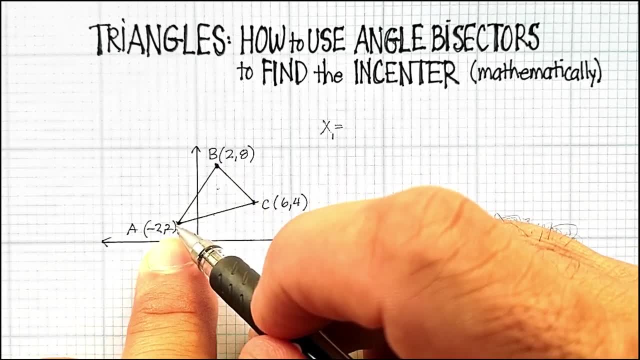 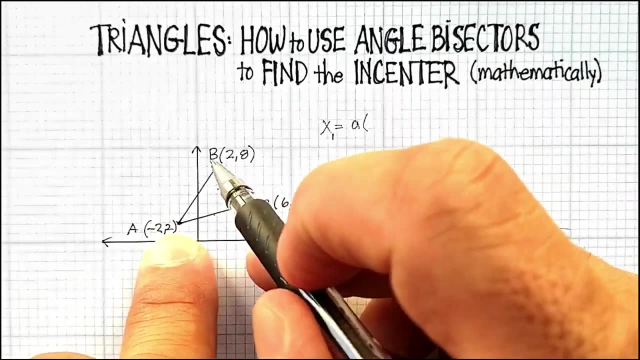 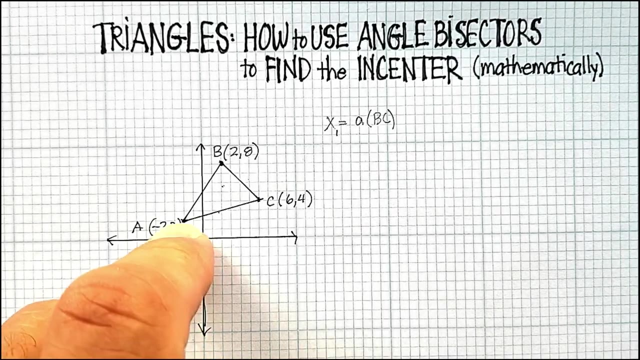 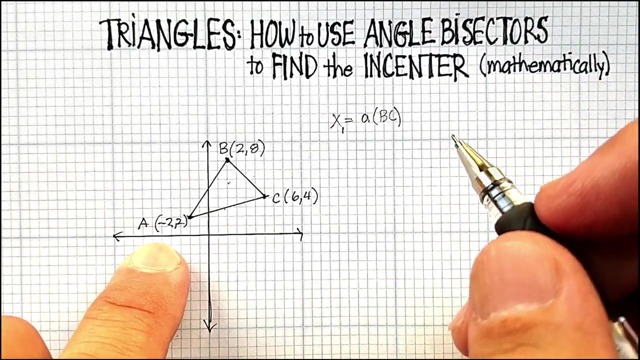 the x value here, which is negative, 2, times the length of the opposite side. Okay, so I'll say that is a times the length of bc. Actually, give me one second here. I need to change my pen. So that is again, it's the a value here, the x value here. 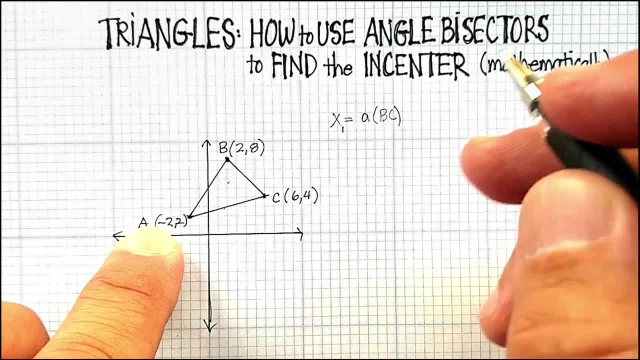 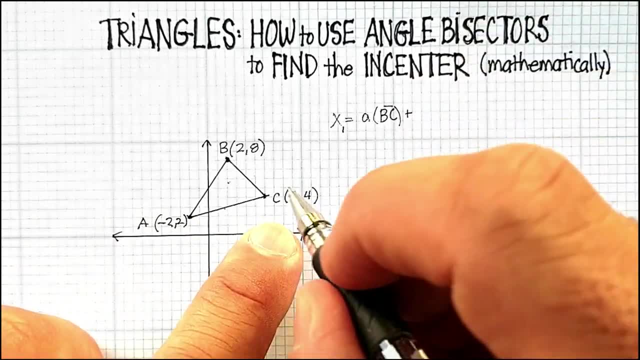 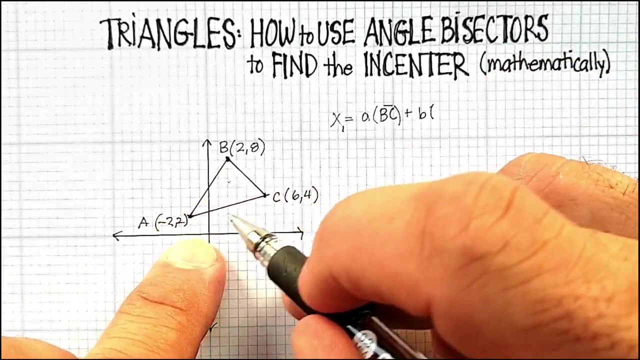 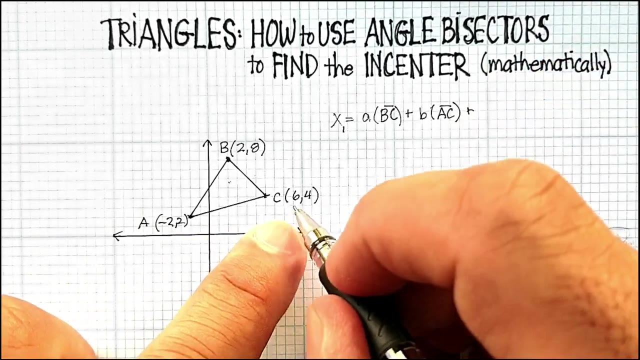 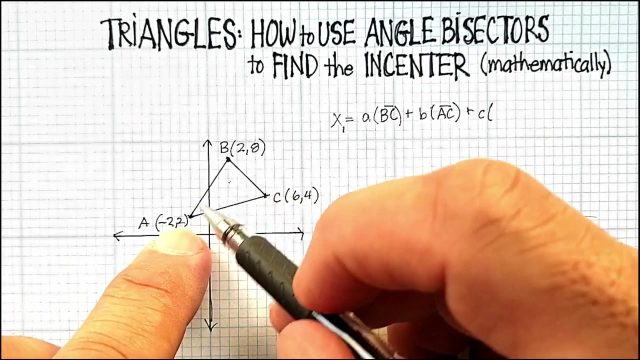 times the length of the opposite side, so times bc, in this case line segment bc plus we'll call this b, small b. the x value there times the length of the opposite side, which is ac plus the x value of the c point. we'll call that small c times the distance here of line segment ab. 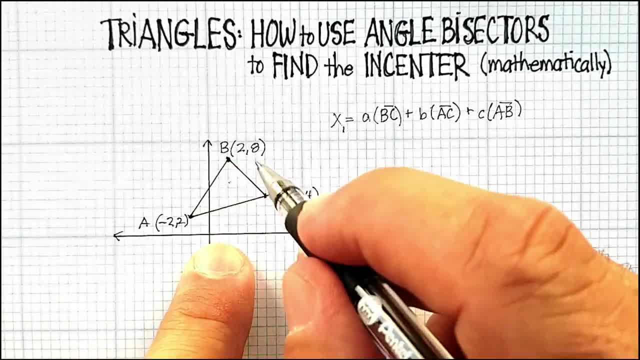 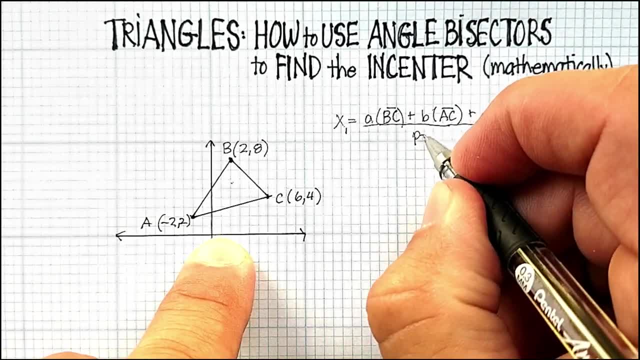 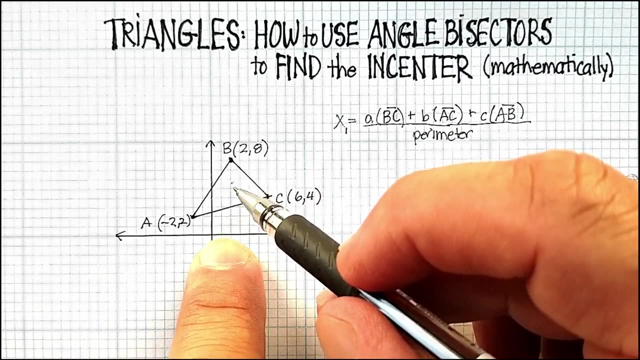 All of that divided by the perimeter of the triangle itself. Okay, so let me just go ahead and draw that line divided by the perimeter. That would be the x coordinate, the x point for the coordinate in the middle right. And we do. 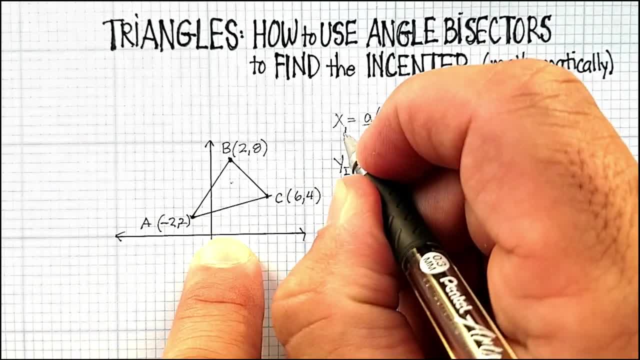 the same thing with the y. The y of the in-center- let me just make that a little bit more obvious- is going to be equal to the y. The y of the in-center- I'll just make that a little bit more obvious- is going to be equal to the y of the in-center. 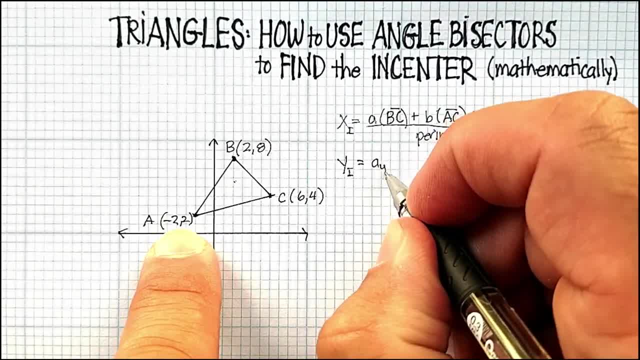 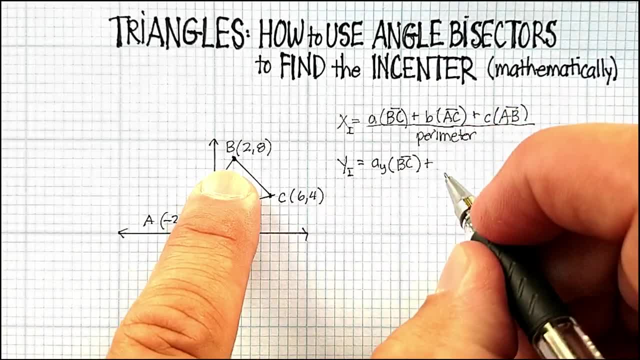 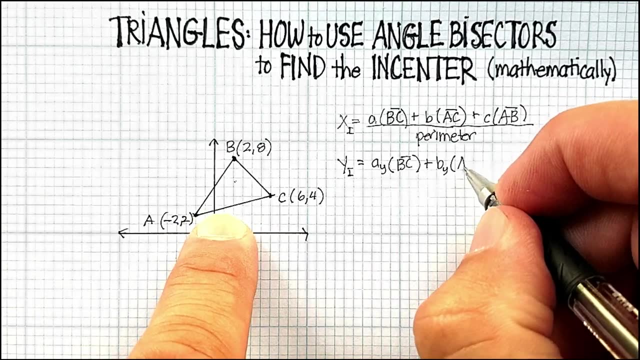 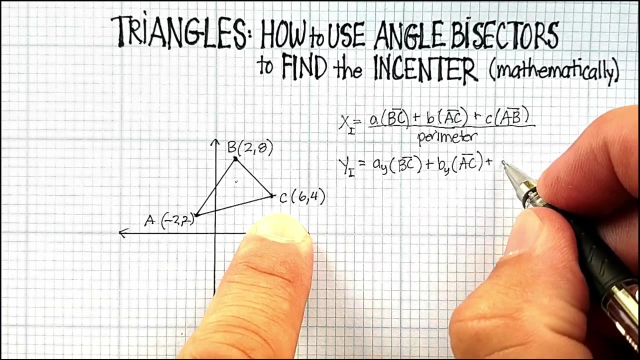 So we'll go a sub y times, again the opposite side, bc plus the b sub y times, in this case ac line segment plus c, the c of the y value, the y value of c, I should say times the opposite side, which is ab. 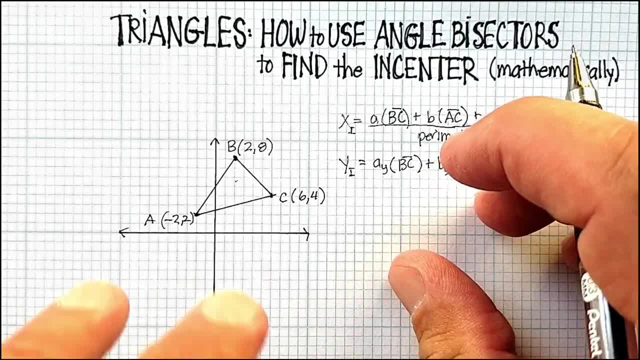 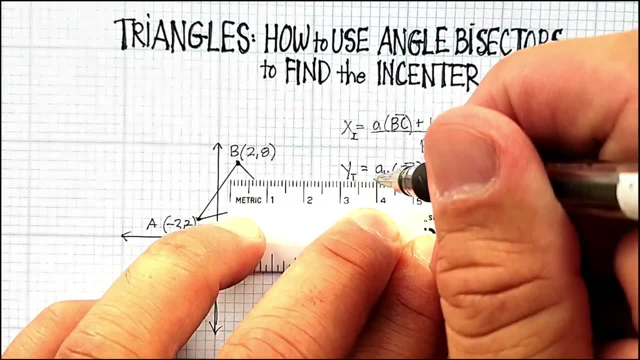 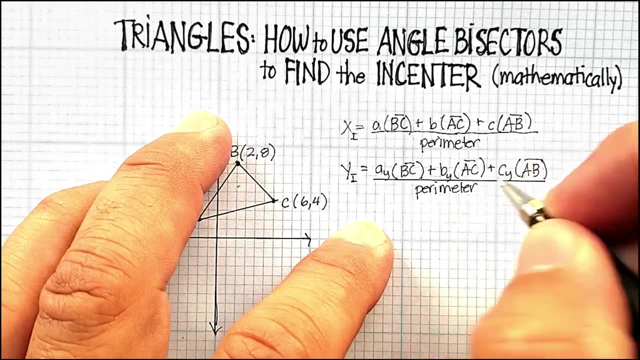 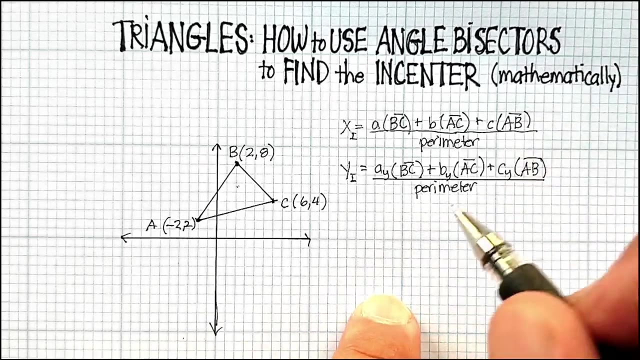 And again, divided by the perimeter. Let me just do this: get a better line this way. Okay, by the perimeter. And that, basically, is the formula to find the in-center. We could do it really quickly for this. let's go ahead and give it a shot. So, again, the first thing I would do: 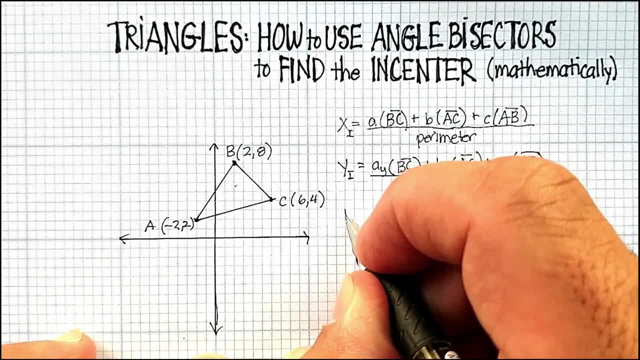 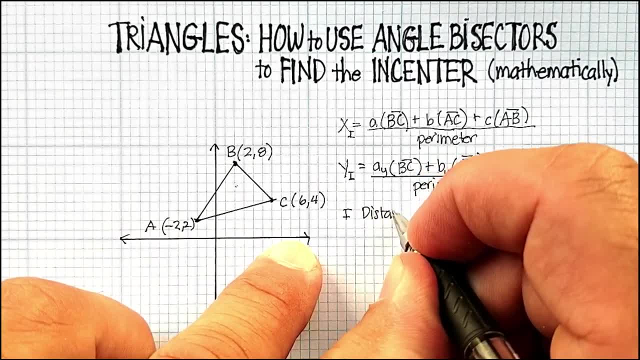 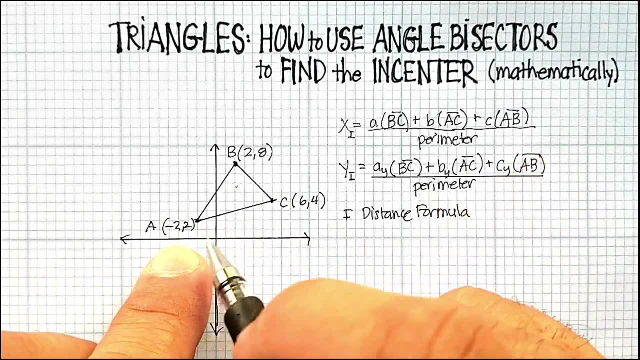 in terms of organizing. my problem is: I'm going to find the power distances of each of the sides of this triangle right, So I'm going to use the distance formula to find each one of the sides of my triangle. So triangle or. 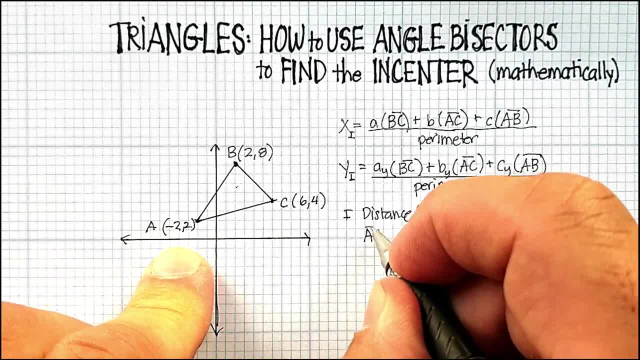 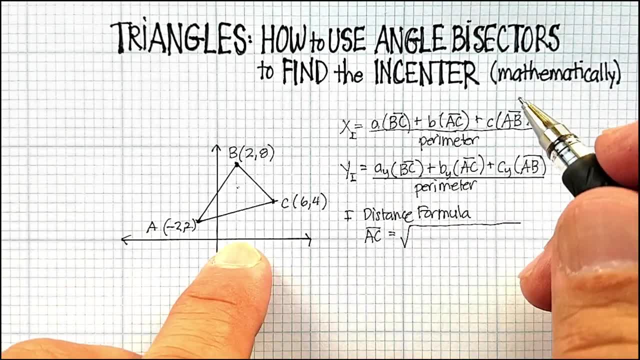 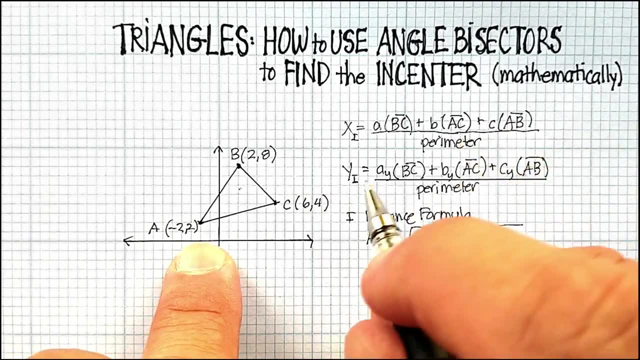 excuse me, side AC is equal. to remember, the distance formula is x1 plus x2 divided by x1 minus x2, quantity squared plus y2 minus y1, quantity squared right. So I'm going to say 6 minus a negative 2. 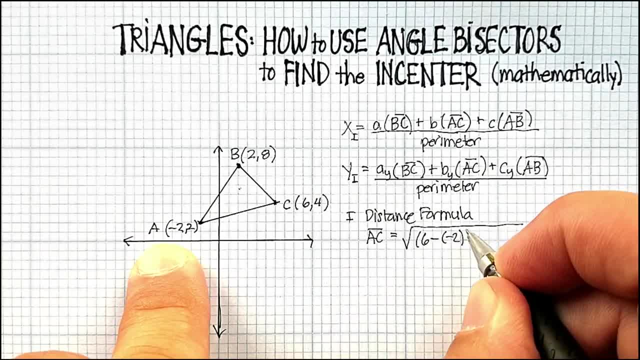 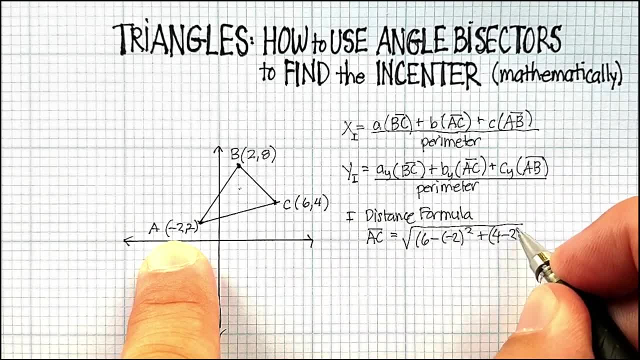 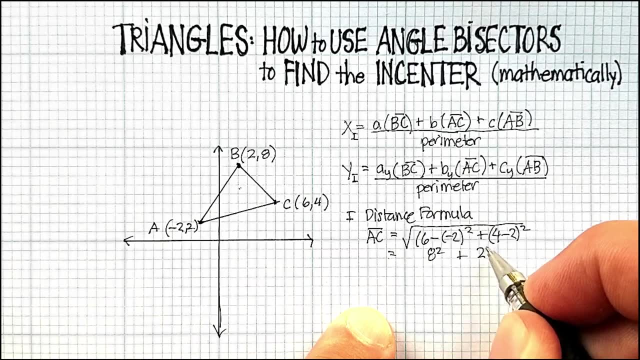 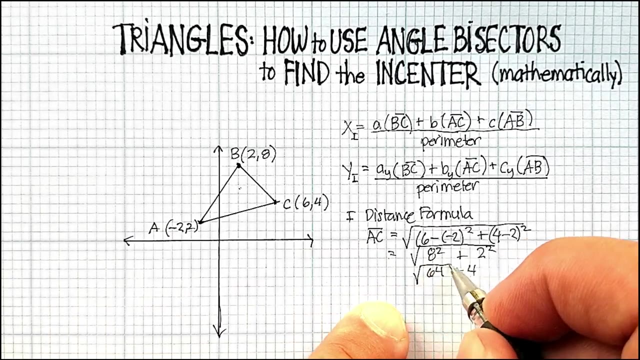 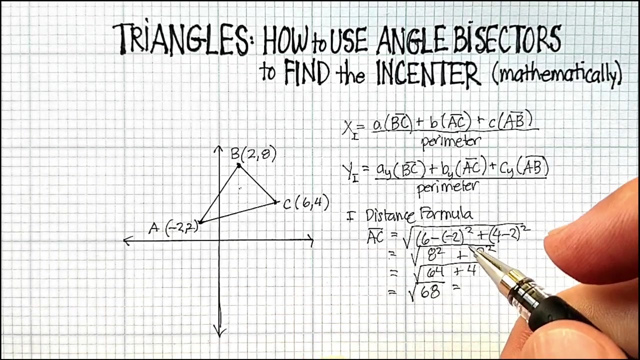 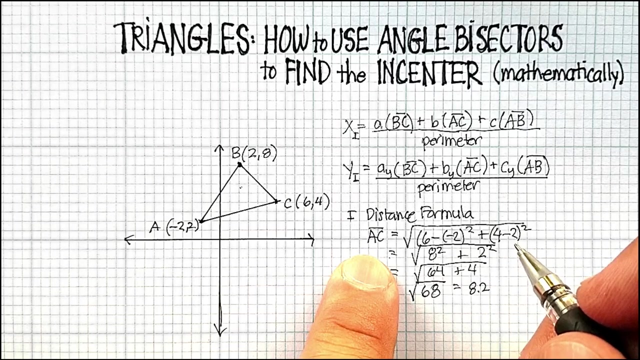 quantity squared plus 4 minus 2. quantity squared, That's going to give me 8 squared plus 2 squared, That's going to give me 64 plus 4, or the square root of 68.. And the square root of 68 is actually approximately 8.2, and that's for side AC. So let's just 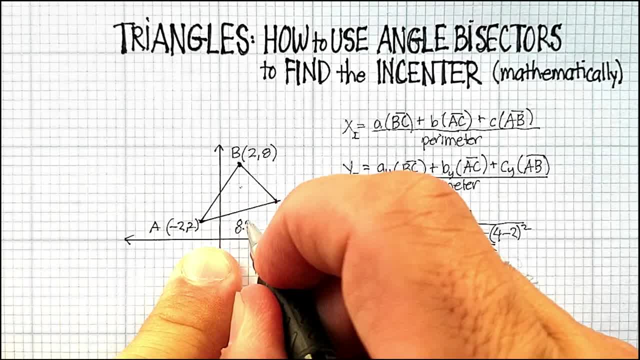 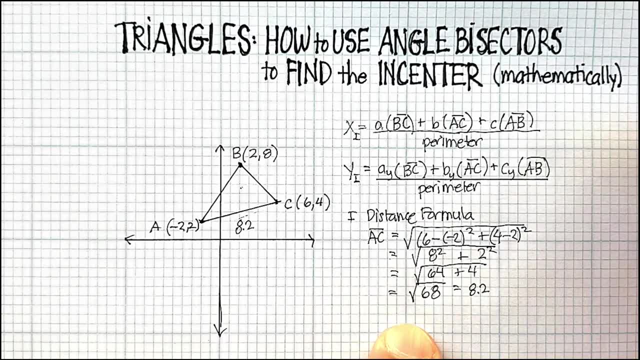 go over here and I'm going to put in 8.2 for that distance. Now I already calculated the other three sides and I'm just going to put them in here, or this video is going to get really long, Okay, but you just basically follow the. 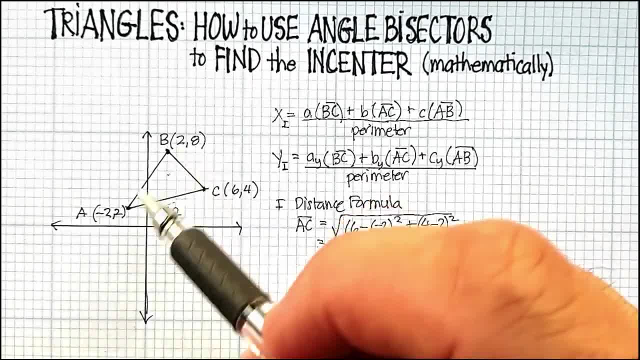 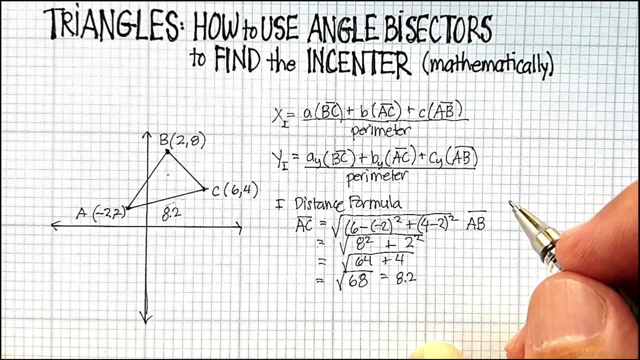 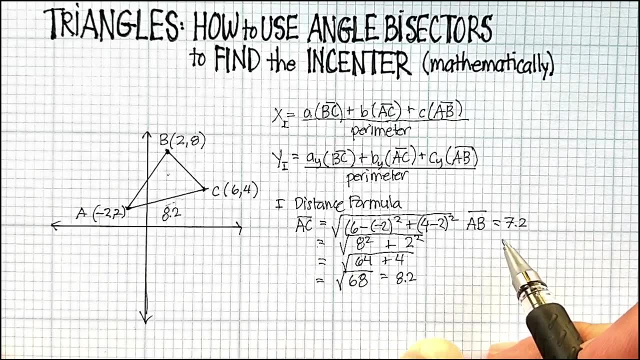 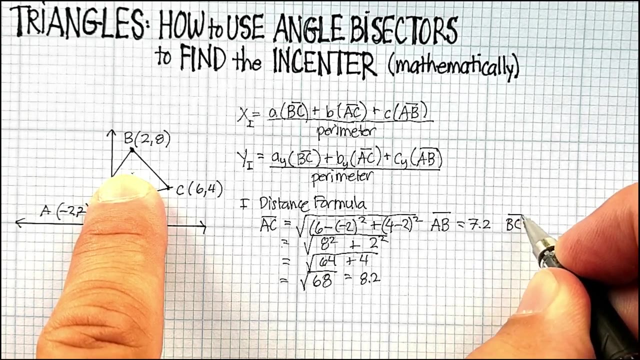 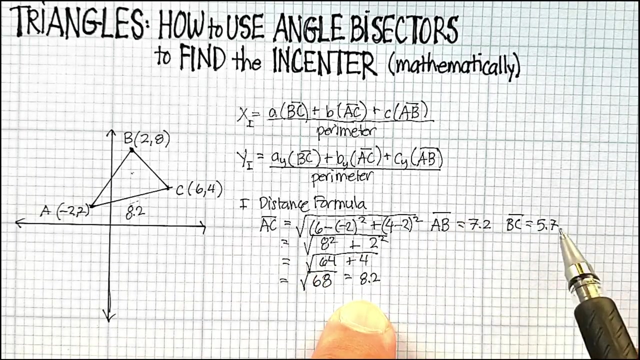 distance formula. all right for AB and AC, And the distance that I found for AB is- let me just quick look- 7.2.. You can go ahead and do your own calculations and see if it matches up to mine. And then the distance for BC I found to be 5.7.. When I added up all three of these distances, 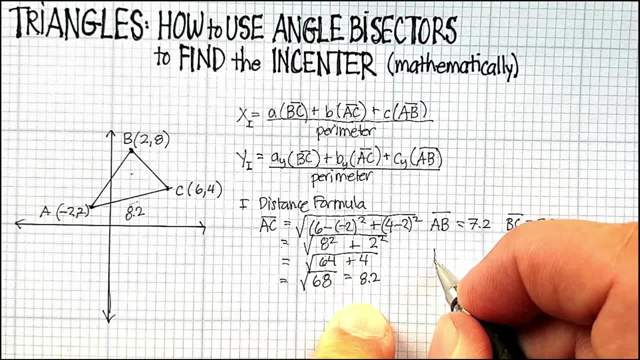 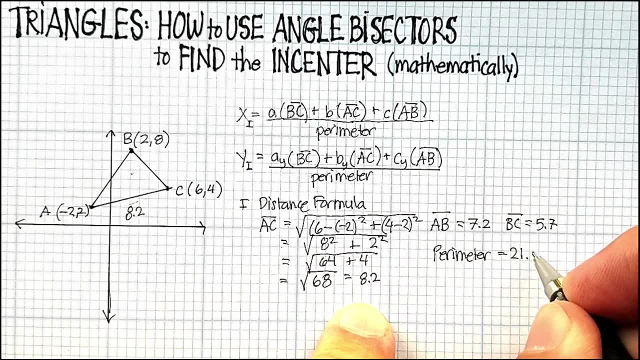 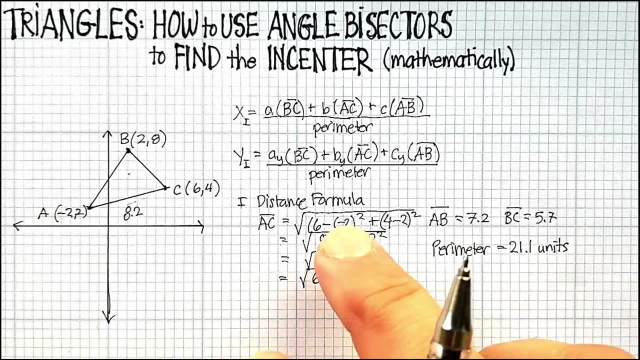 I got 21.. The perimeter is equal to 21.1 units. okay, And I'll just put units here. Okay, so now that I've got the perimeter, let me just go ahead and do the x value And you can see. 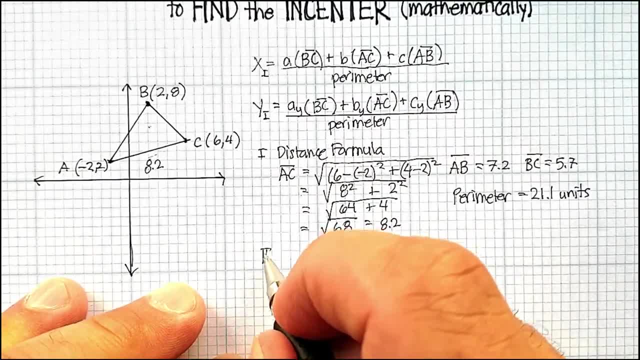 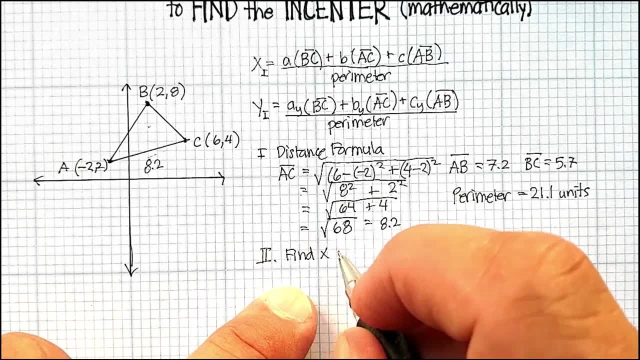 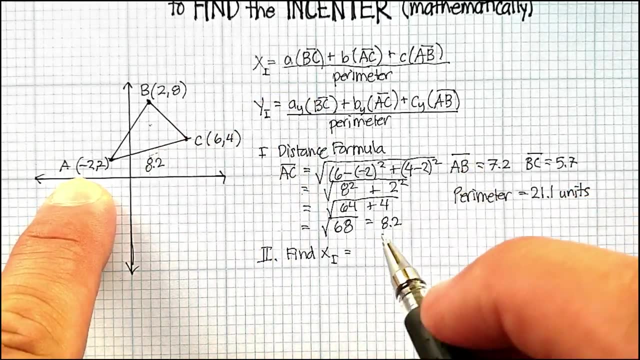 how that works. So let's find the x, So that'll call. we'll call this 0.2.. Finding the x of the in-center: Again, we said that was equal to negative 2 times the opposite side, which in this. 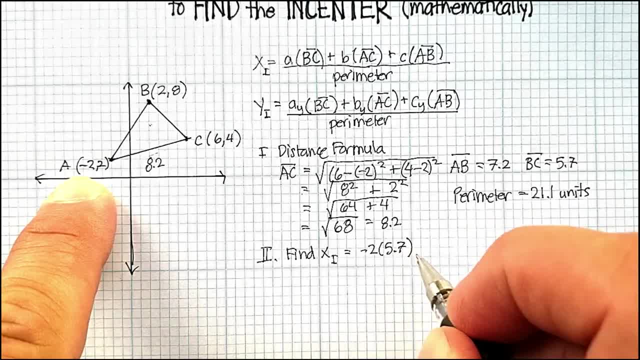 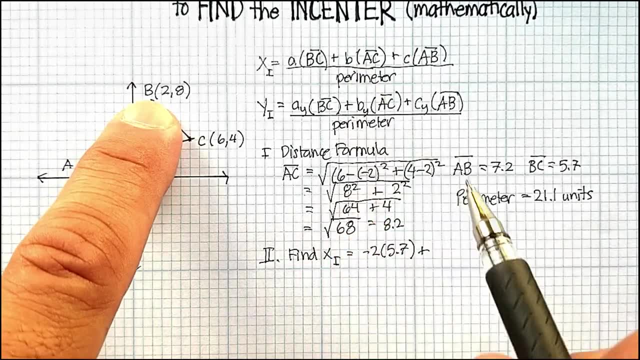 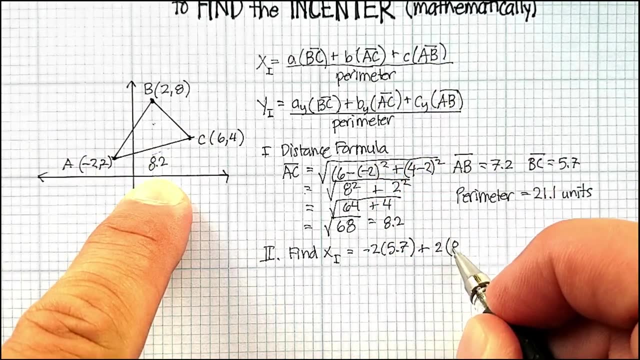 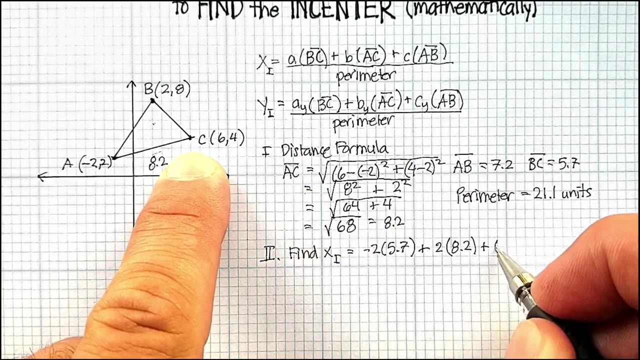 case would be BC, So 5.7 plus value of B, which was x of B, which is 2 times the opposite side which is AC, which is 8.2, plus the x value for C, which is 6 times the opposite side of, or, in other words, just AB Did. 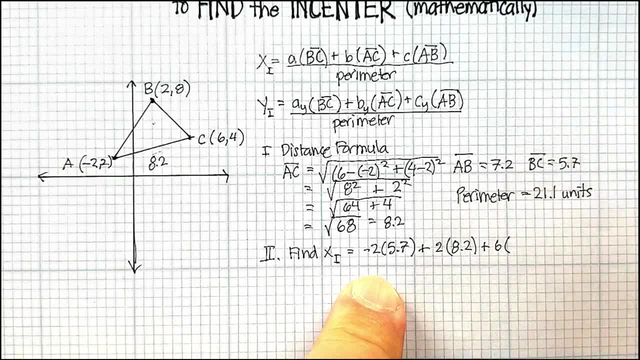 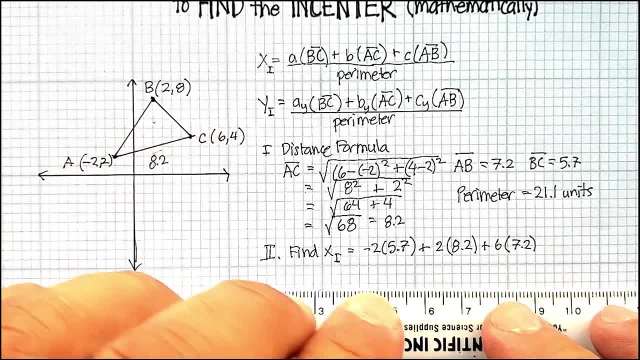 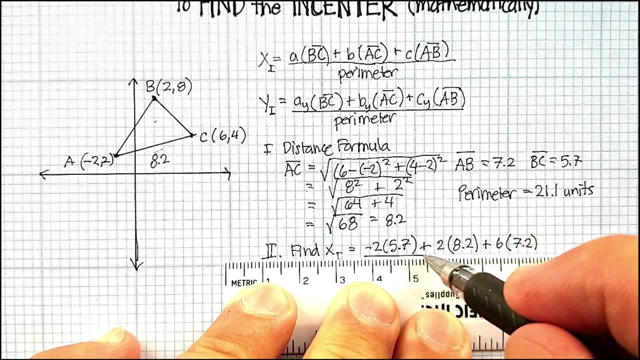 I do that right, I think I did, And AB I said was 7.2. All divided by 21.1, which is the perimeter that I just figured out in the previous, what I'll call paragraph- okay, This is a mathematical paragraph- Divide by 21.1.. 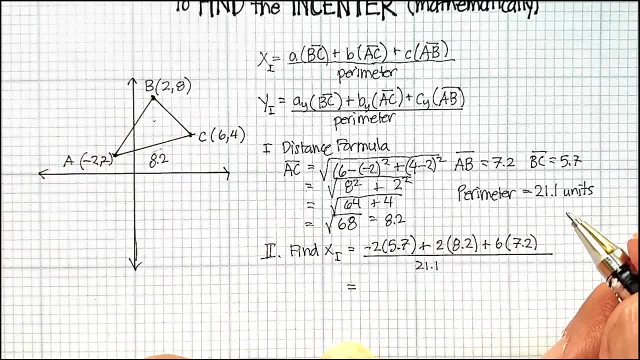 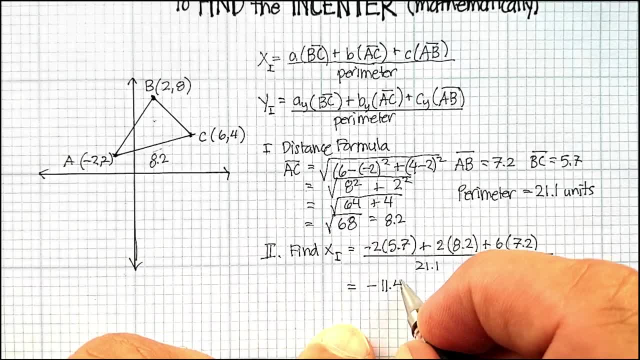 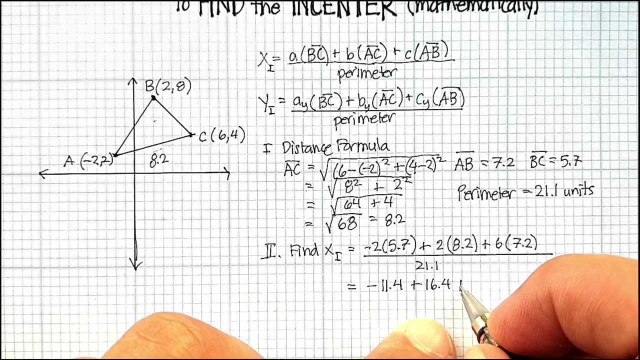 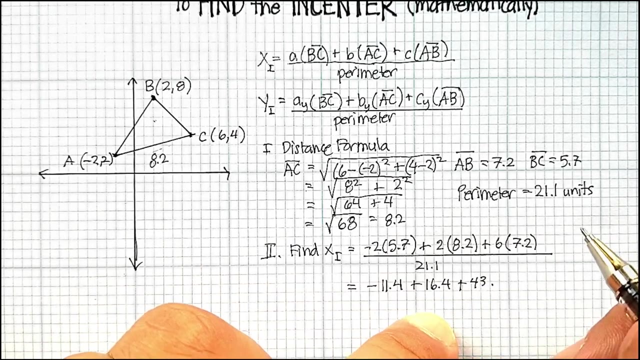 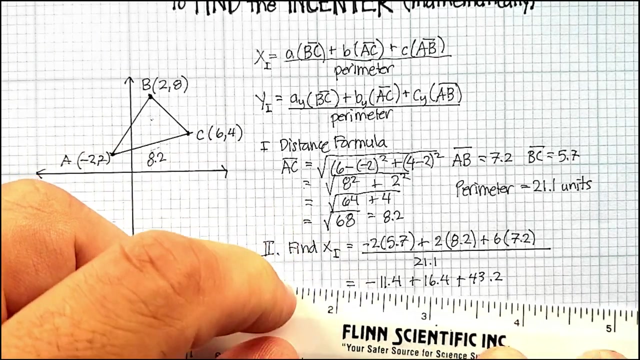 I'm going to add all that up and let me see what do I get. That's a negative 11.4.. That's a negative: 16.4.. That is a positive 43.2.. Yeah, Yeah, 43.2.. Divide by 21.. And again: 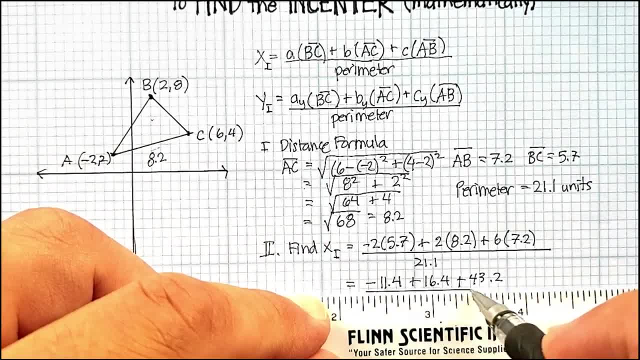 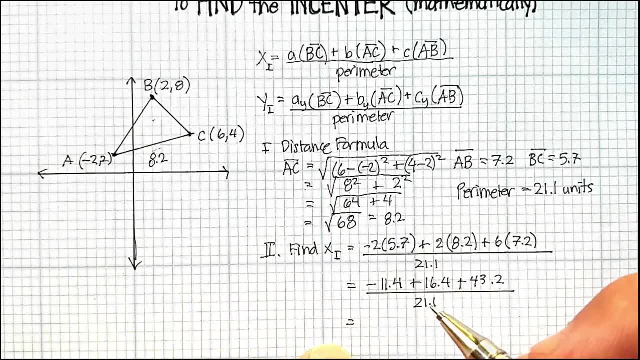 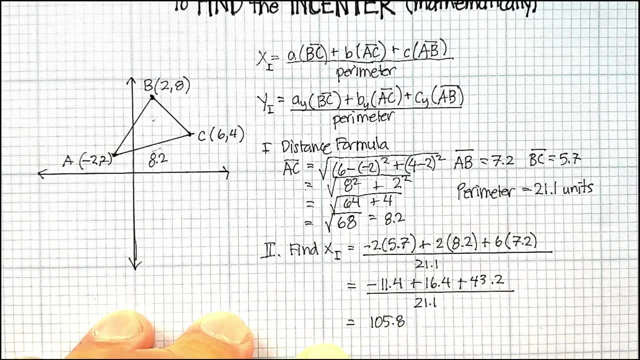 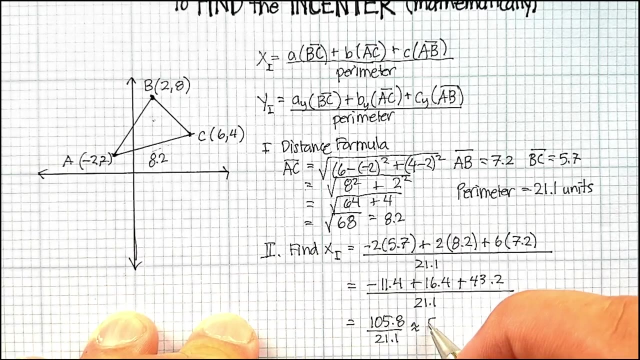 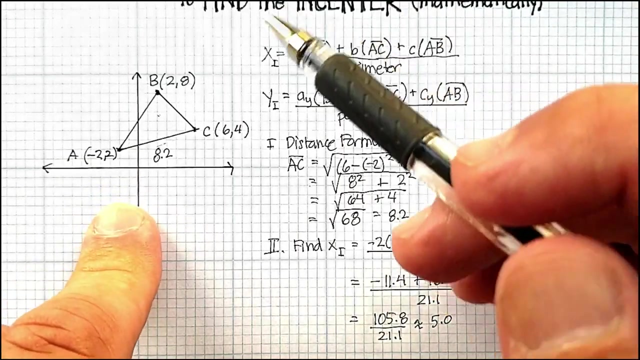 I'm just going to do this quickly. You can do the calculations on your calculator And it turns out that my x value for my in-center turns out to be 105.8 over 21.1, or 5.0.. Now let me just go to my actual triangle. okay, And I eyeballed it. 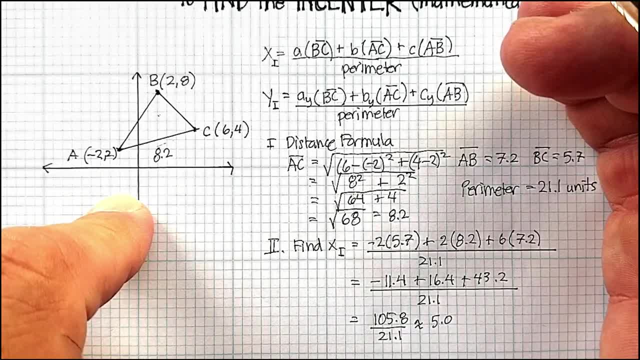 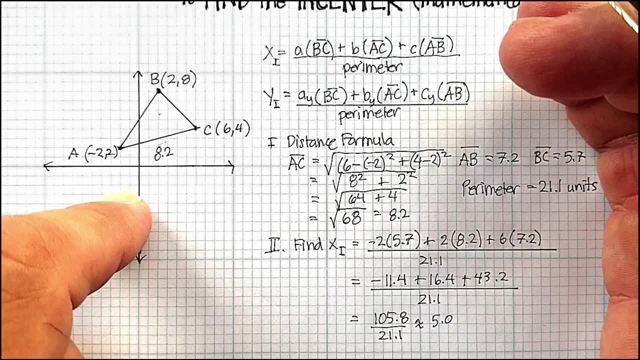 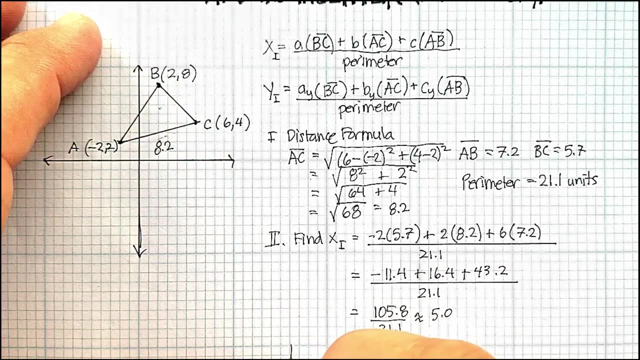 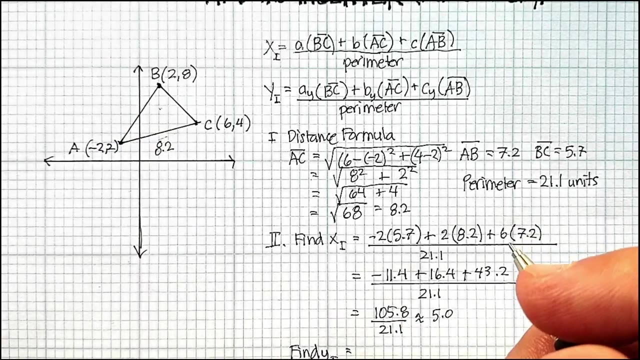 Correctly, I believe, Did I? Yeah, That still sounds okay. Now let's find the y value, okay, The y of the in-center, And I'm going to tell you that, after I did all my calculations, so 2 times this opposite side. 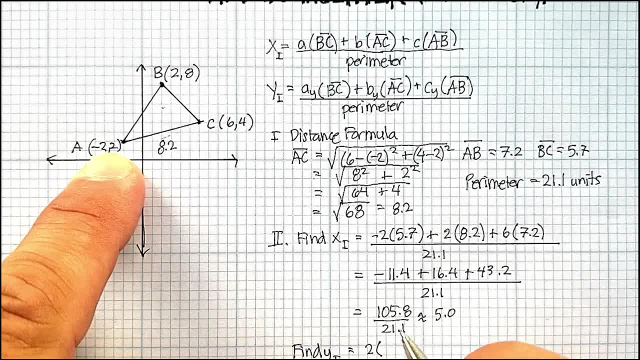 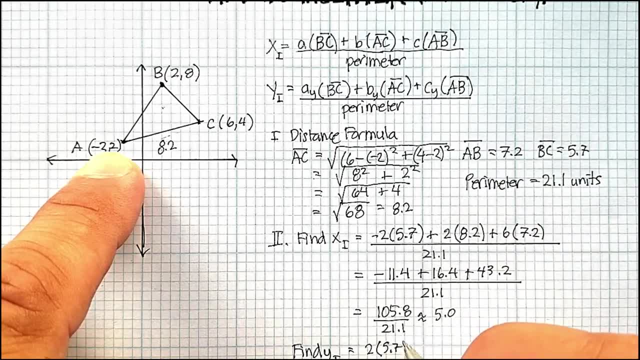 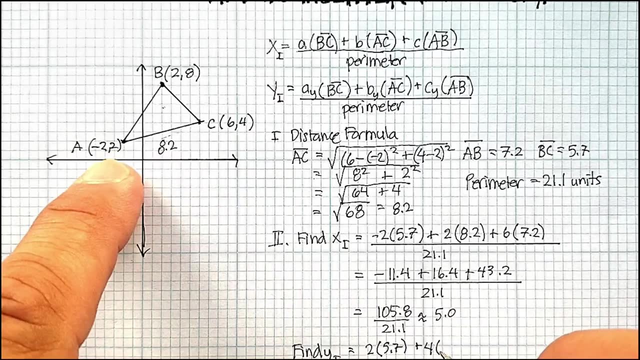 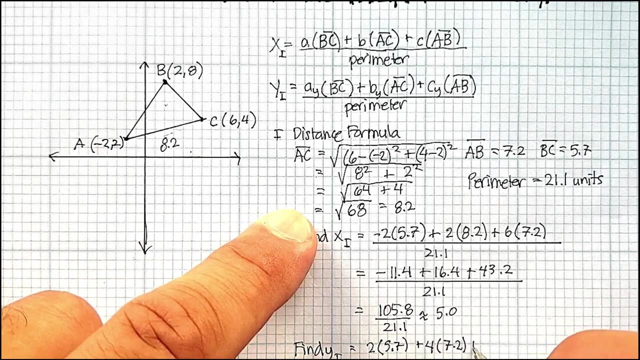 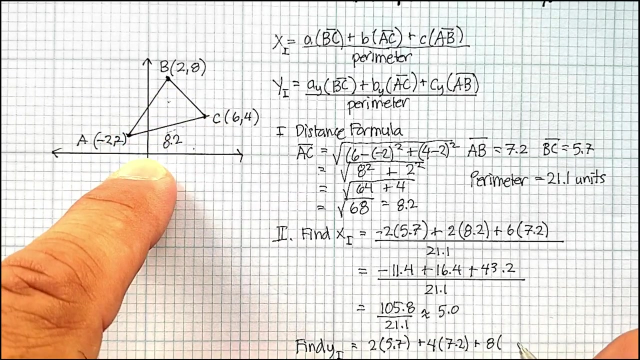 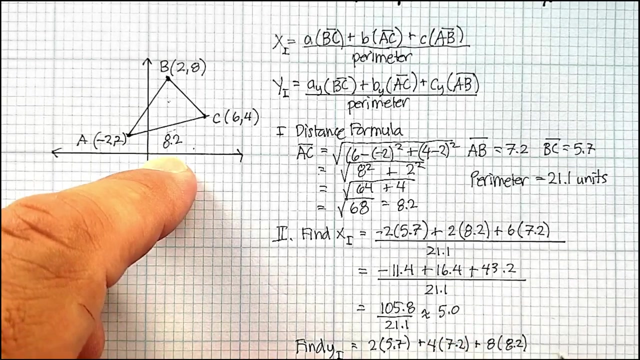 2 times bc. And what did I come up with? bc was 5.7 plus 4 times ab, And we said ab was 7.2 plus 8.. The y value Times 8.2. here That's going to turn out to be: oh, excuse me, I see what I did wrong. 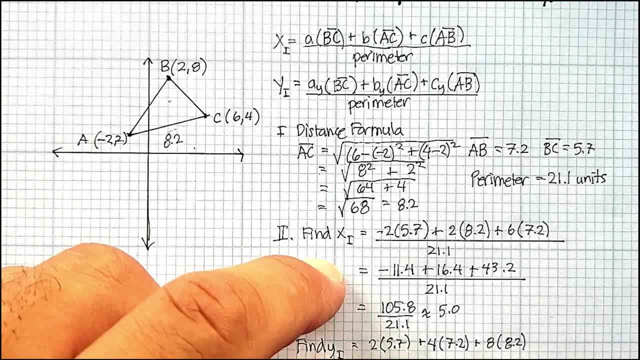 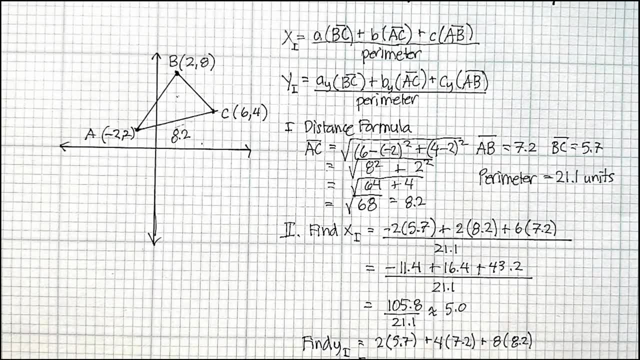 105.8 over 21.8, that's the y value. I was looking at my calculations over here And I added them up incorrectly, So please excuse me for that. That was the y value. Okay, All right.